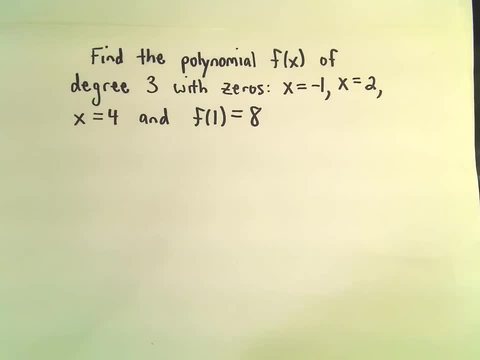 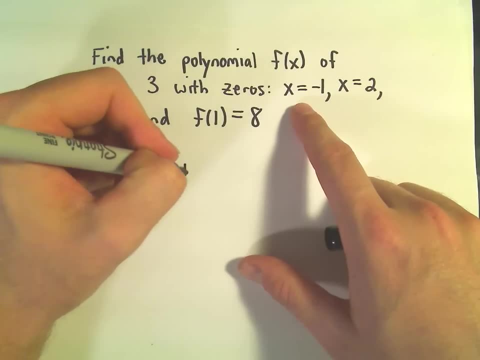 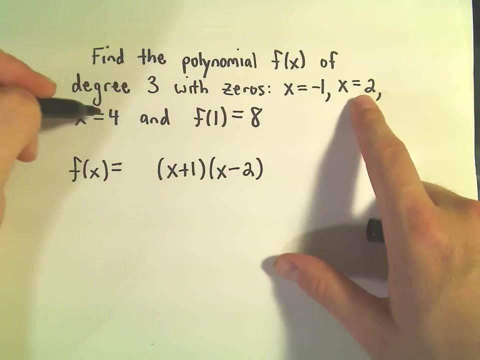 and satisfies this condition that if you plug 1 in, we get 8 out. Okay, so a couple things. Since we know that negative 1 is a zero, that means that x plus 1 is a factor. If x equals 2 is a zero, that means x minus 2 is also a factor. 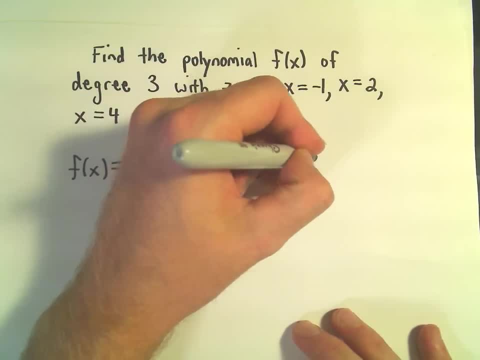 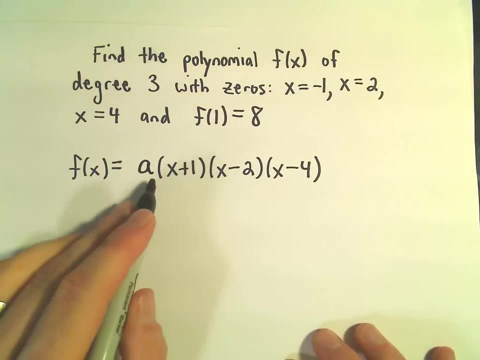 And if 4 is a zero, that means that x minus 4 is also a factor. Okay, now the other thing is we could have some number hanging out front. We'll call it a. That wouldn't change the fact that negative 1,, positive 2, and positive 4 are all zeros. 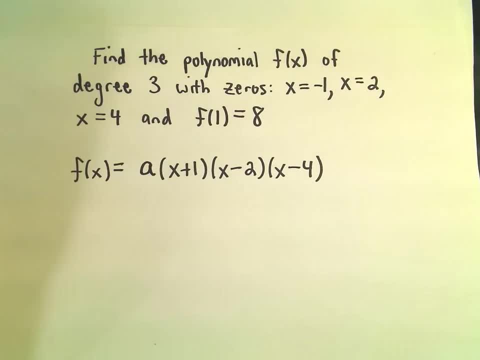 Okay, so basically, at this point, all we need to do is figure out our a value. So I'm going to solve for a by using this formula, By using this extra point. And again, this says: if you plug in x equals 1, it says we get out the y value of 8.. 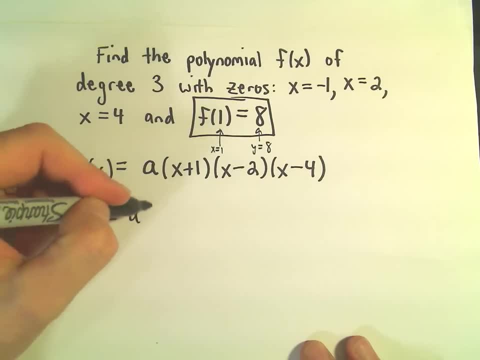 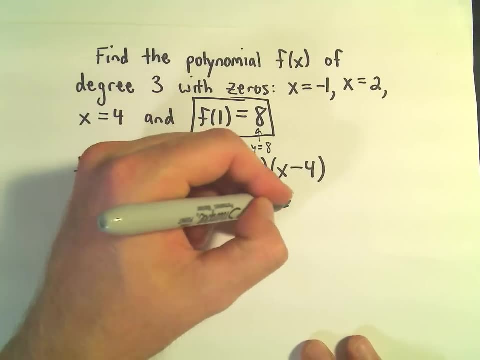 So I'm going to put 8 on the left side And then I'm just going to plug 1 in. everywhere there's an x. So we'll get 1 plus 1, 1 minus 2, 1 minus 4.. 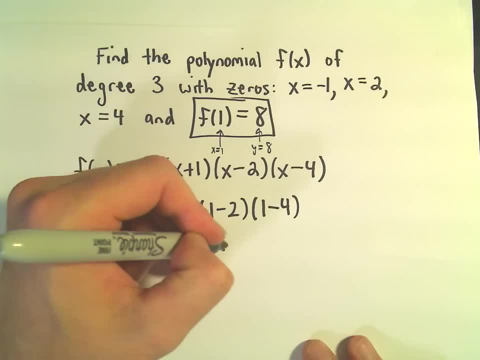 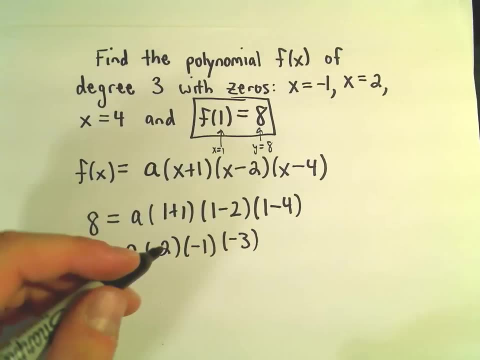 Okay, well, that gives us 2 times negative, 1 times negative, 3.. Well, let's see Negative 1 and negative 3. Or positive 3 times 2 is 6. So we get 6 times a. If we divide both sides, we'll get 8 over 6.. 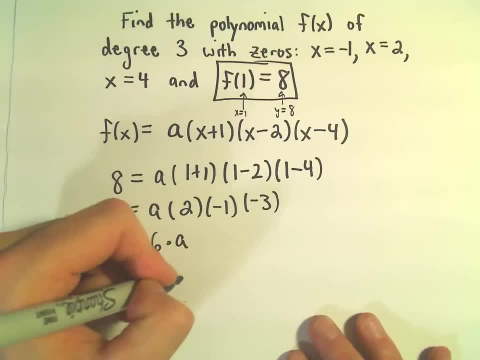 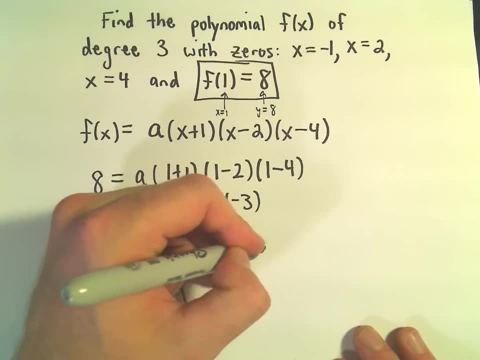 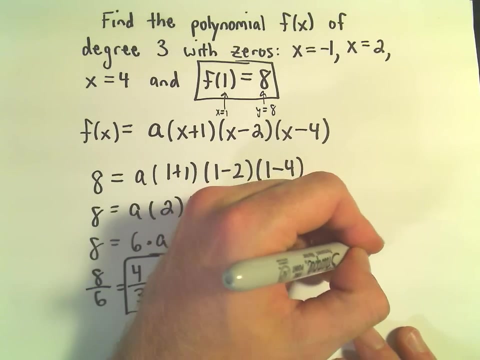 If we divide that by 2, we'll get 4 thirds, And that's going to be our a value. Okay, so it says our polynomial is: f of x equals 4 thirds times x plus 1 times x minus 2 times x minus 4.. 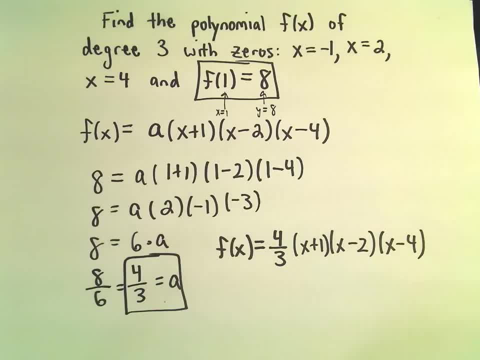 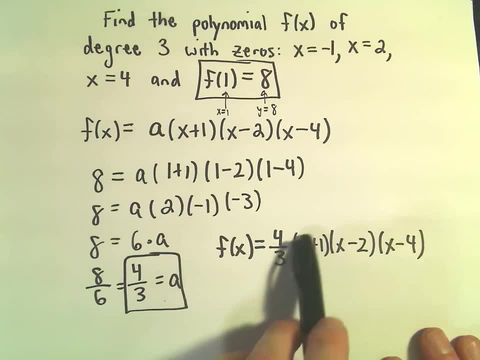 And of course, if you wanted to, at this point you could even multiply all this out, But I'm going to call it a day and leave it right there. This is now our polynomial, with the given zeros of degree 3.. And this coefficient will make it go through the y coordinate of 8 when we plug in: x equals 1..